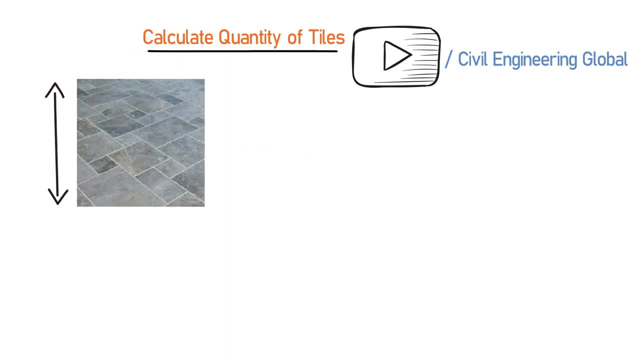 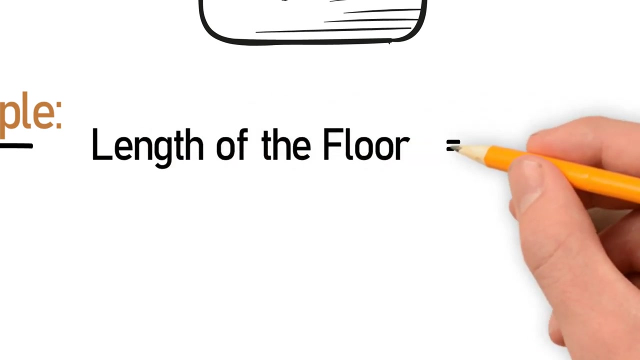 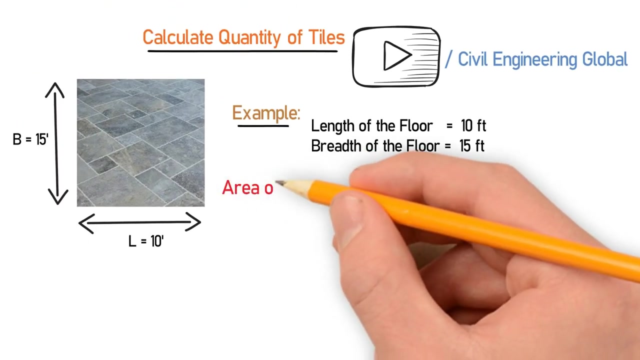 In this example we have: the breadth of the floor is 15 feet and the length of the floor is 10 feet. So the length is 10 feet and the breadth is 15 feet in this example. So we have the following data: Length of the floor: 10 feet, breadth of the floor: 15 feet. So first we have to 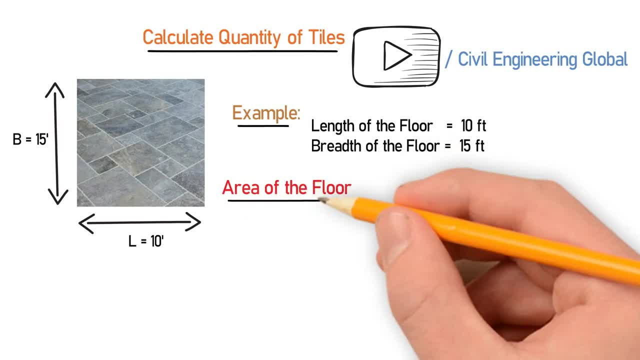 calculate the area of the floor. So how much is the total area of the floor? For this purpose, we have the formula: area is equal to length multiplied by breadth. So this will become 15, which will give you 150 square feet. So this is the total area of the floor. So as 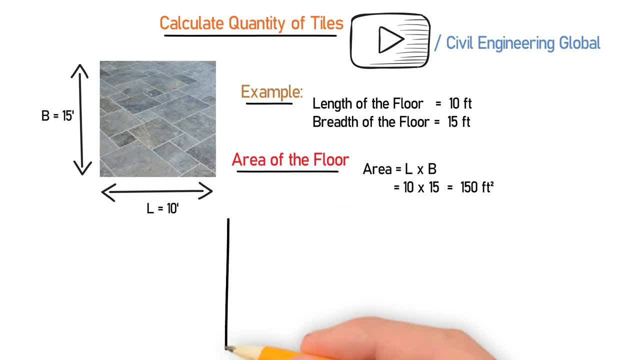 we all know that the size of the standard size of one tile- So the size of one tile- is the length is 2 feet and the breadth is 1.6 feet. So let's calculate the area of one tile. The above was the area of total floor and this will be the area of one tile. So this 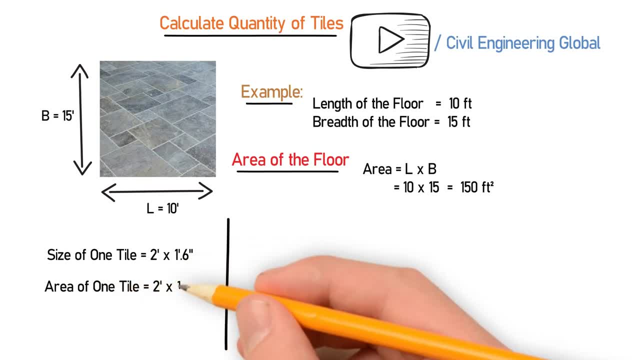 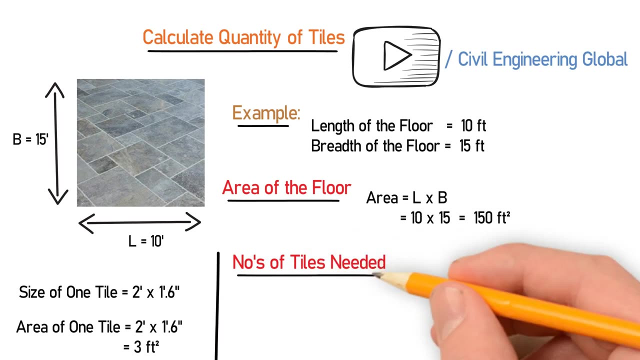 will become. area of one tile is equal to 2 multiplied by 1.6, which will give you 3 square feet. So this area of one tile is 3 square feet. So now let's calculate the number of tiles needed for this floor. So how much, how many number of tiles will be required? 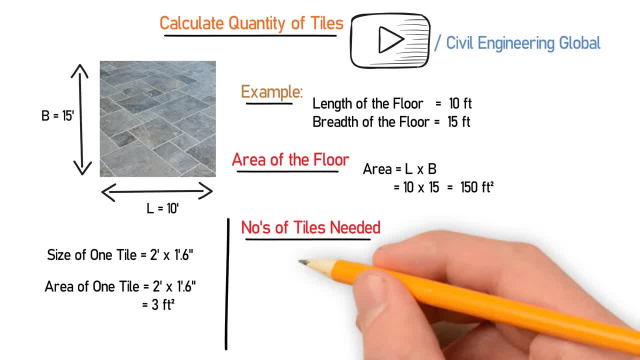 for this floor. For this we use the formula: number of tiles is equal to total area of the floor divided by area of one tile. So total area of the floor we have calculated, which is 150, and area of one tile, which is 3.. So 150 divided by 3, this will give you 50. So this means